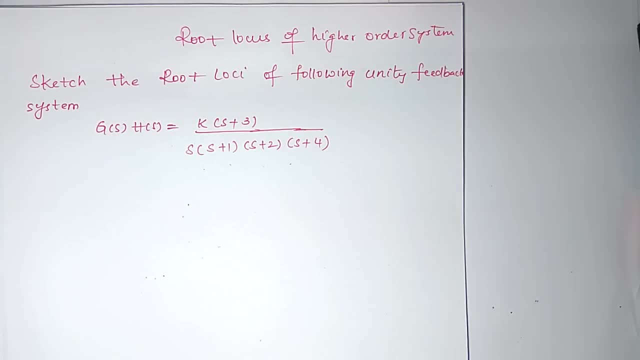 Next is root locus of higher order systems. So let's plot the root locus for the given open loop transfer function. So given open loop transfer function is G of S into H of S is equals to K into S plus 3, by S into S plus 1, into S plus 2 and S plus 4.. The first 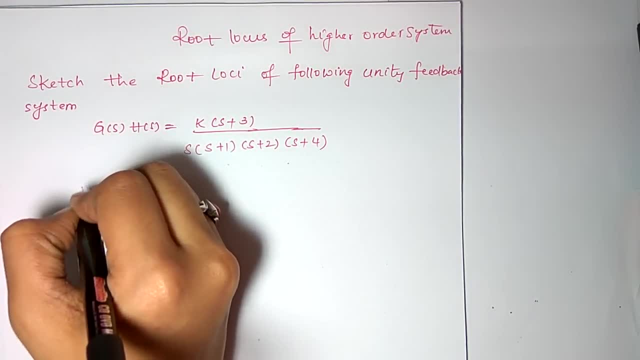 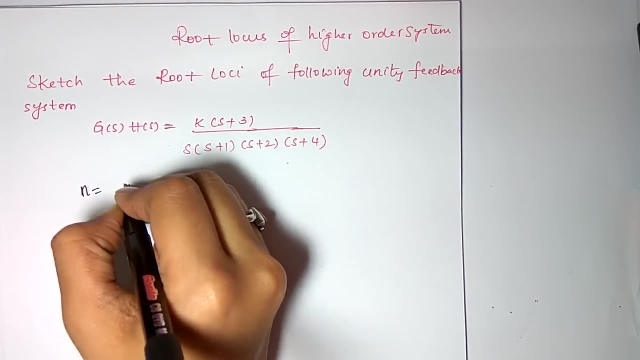 thing is number of poles. Number of open loop poles N is equals to 1,, 2,, 3,, 4. 4 open loop poles and number of open loop zeros is 1.. So number of azimutodes. suppose azimutodes. 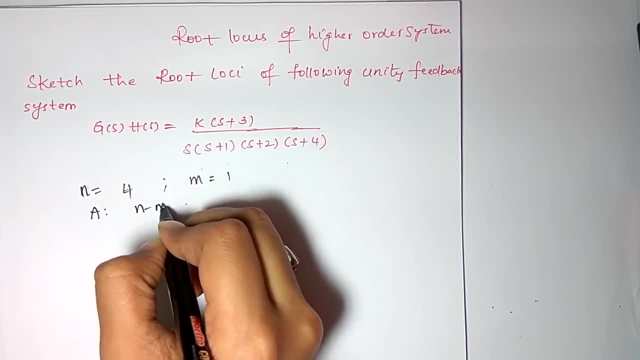 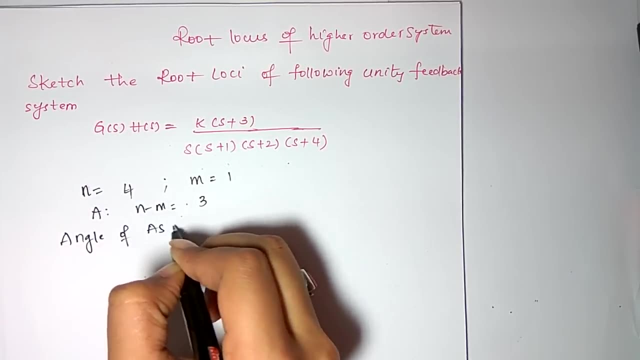 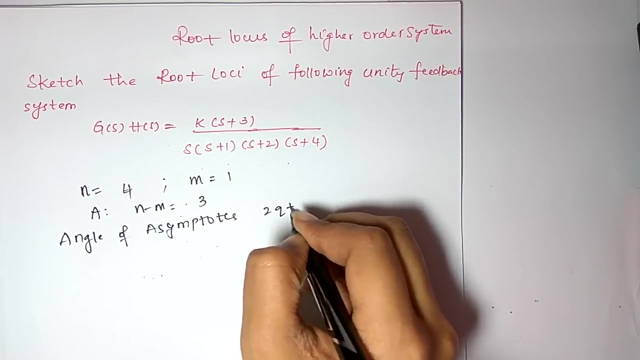 A denoted by A is equals to N minus M is equals to 3 and angle of azimutodes: angle of azimutodes is equal to N minus M, Is equals to 2Q plus 1, by n minus m into pi. 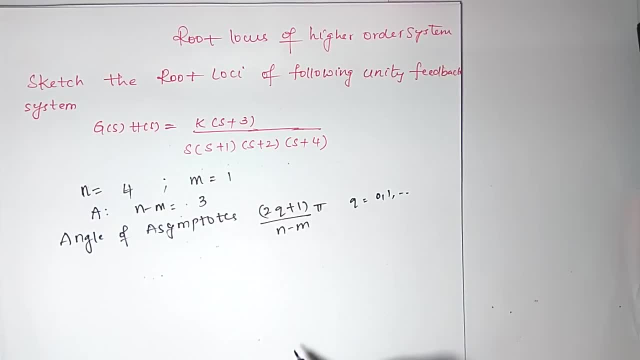 Where Q is from 0 to 1 to n minus m minus 1.. n minus m is 3.. So n minus m minus 1 will be 2.. So when Q is equals to 0, it will be pi by 3.. 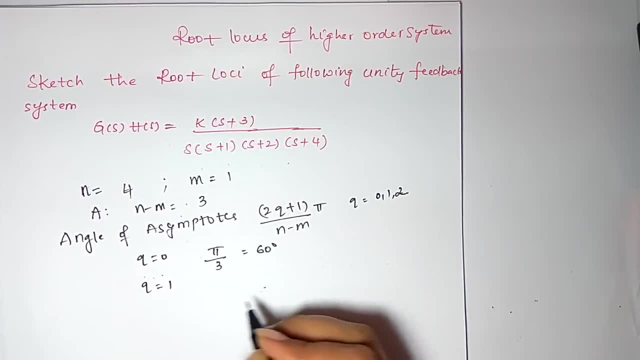 That is 60 degrees. When Q is equals to 1, it will be 3 into pi by 3, which is 180 degrees. When Q is equals to 2, it will be 5 into pi by 3, which will be 300 degrees. 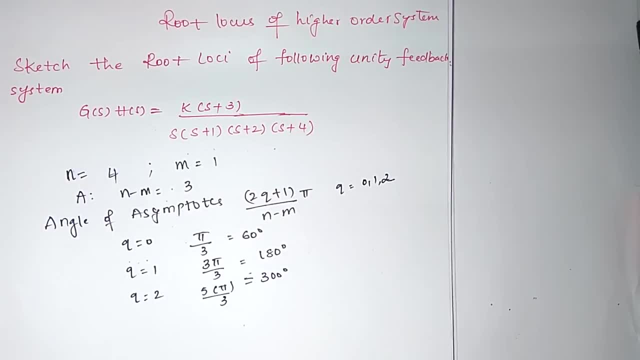 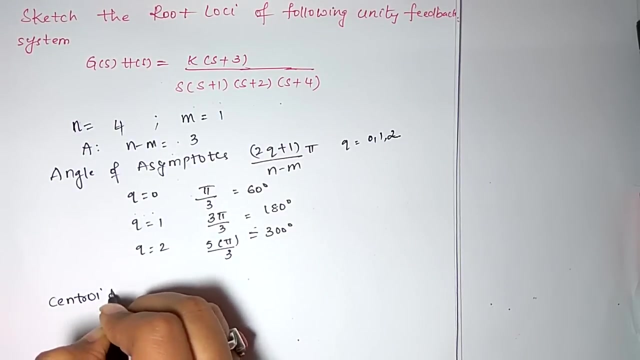 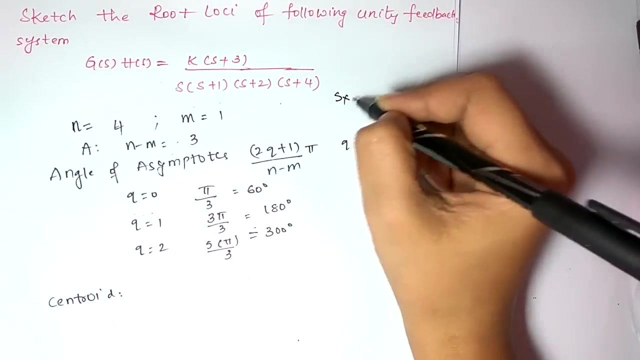 So angle of azimuthal is 60 degrees, 180 degrees and 300 degrees And find the intersection point Centroid. Centroid is equals to sum of poles. Poles are, I am denoting by s poles s cross, 0 minus 1 minus 2 minus 4.. 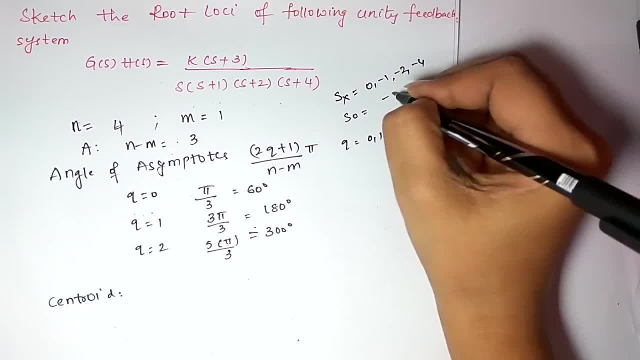 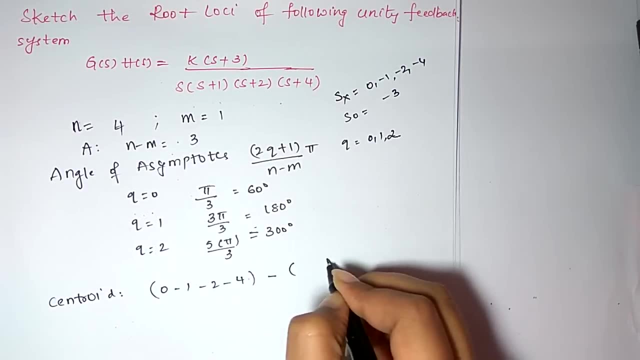 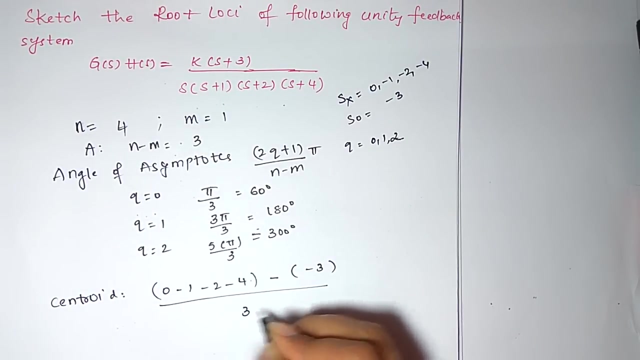 Whereas zeros with s: 0 minus 3.. Sum of poles: 0 minus 1 minus 2 minus 4.. Minus sum of zeros: minus 3, only 0 by n minus m. n minus m is 3.. So which will be equals to minus 1 minus 2 minus 3, minus 7 plus 3 minus 4 by 3.. 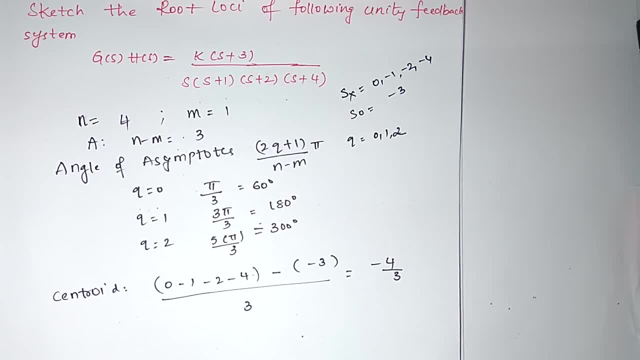 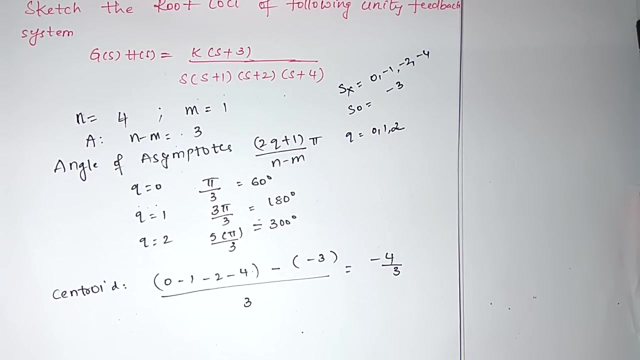 So centroid, All the azimuthals will intersect at the point minus 4 by 3.. Next Draw the right Rough sketch of the root locus. that means first plot the mark, the poles and zeros. So this is the j omega axis and this is the real axis. 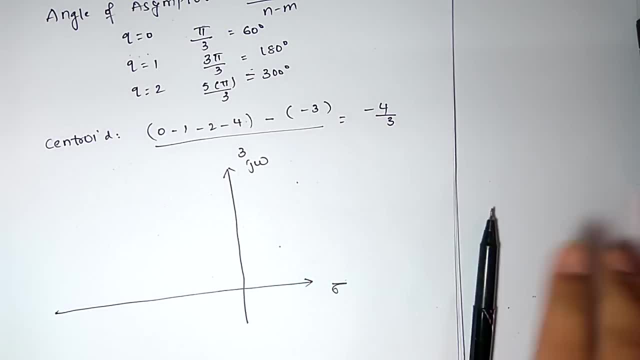 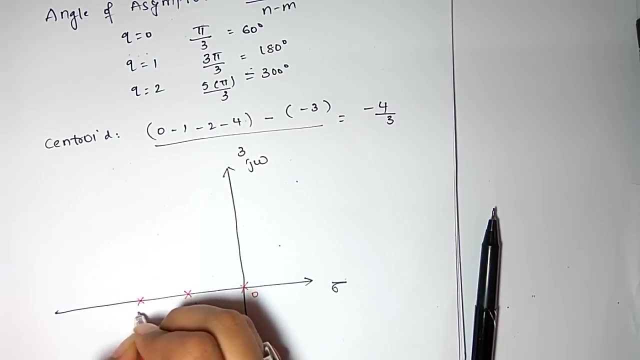 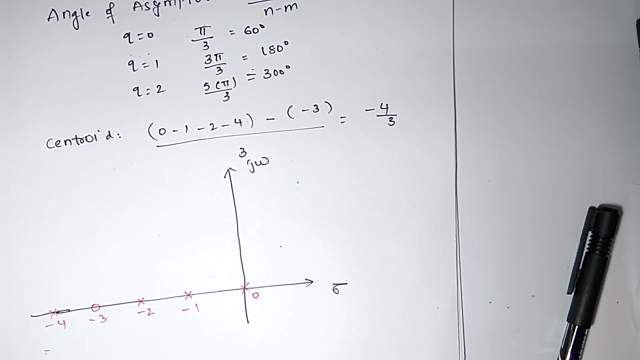 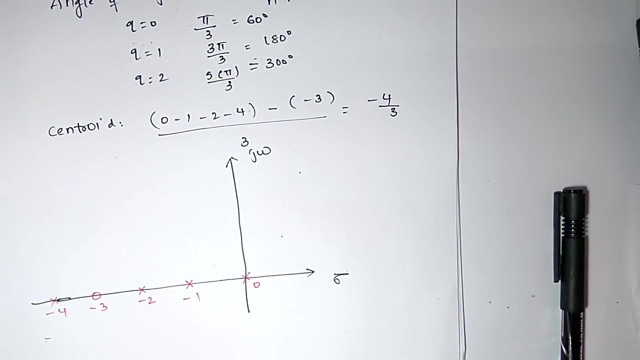 So first mark the poles with cross: 0 minus 1 and minus 4.. Sorry, 0 minus 1 minus 2.. 3 is 0 and the 4 is a pole. this is a pole. so this is the next draw, the azimuthals. and what is the intersection point of azimuthals minus 4 by 3? that means it will lies between minus 1 and minus 2, almost near to 1.. 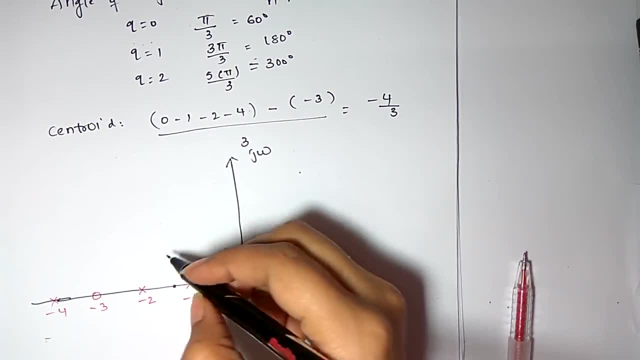 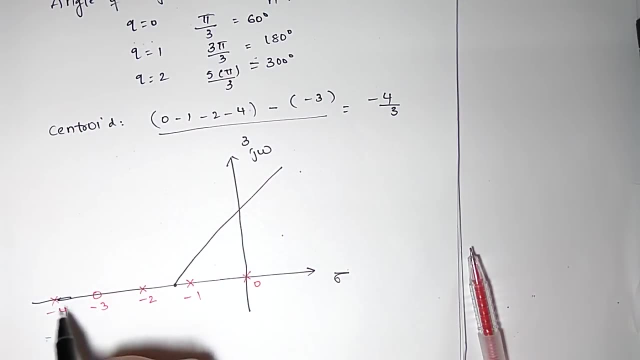 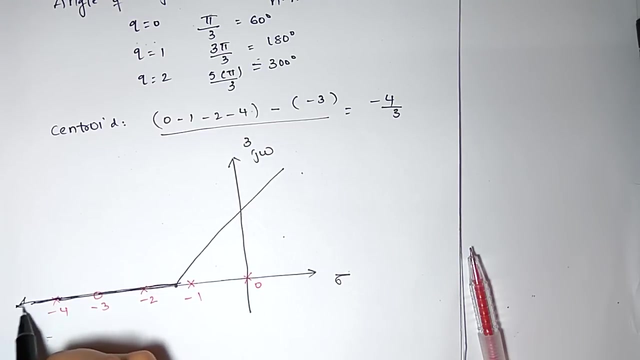 Suppose this is the thing plus 60 degrees. This is the plus 60 degrees azimuthals and 180 degrees azimuthal. So 180 degrees azimuthal means this one Don't think it is not a root locus. This is the azimuthal. 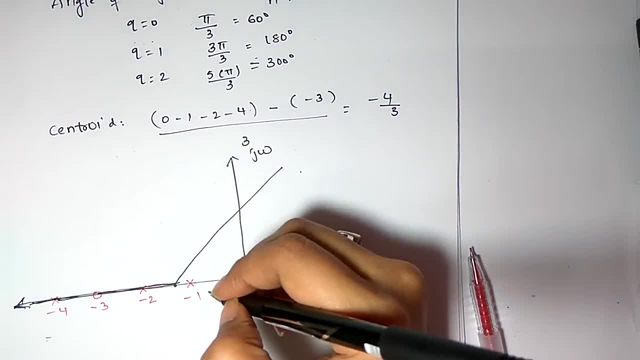 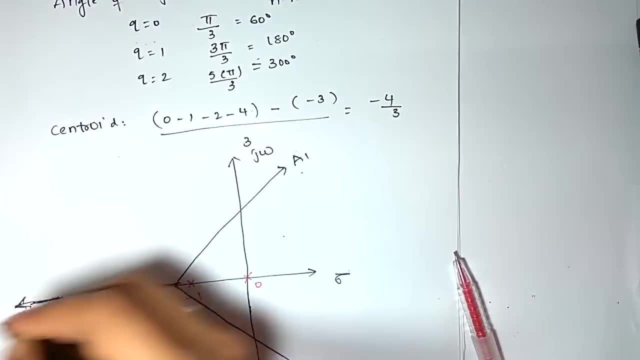 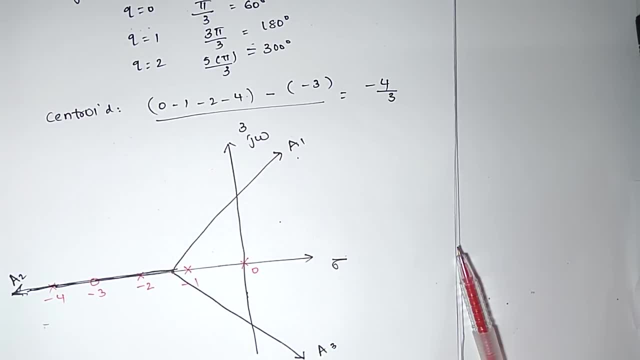 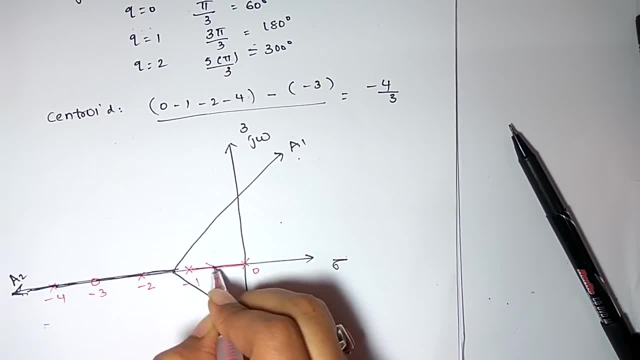 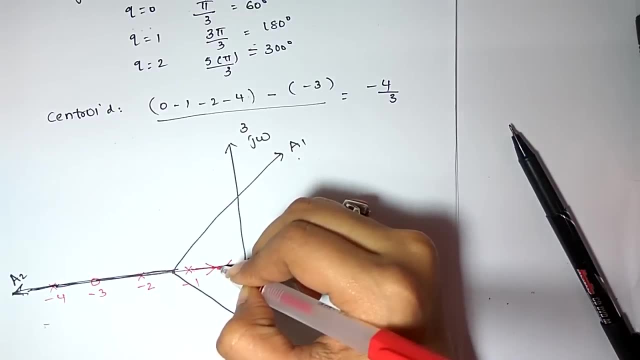 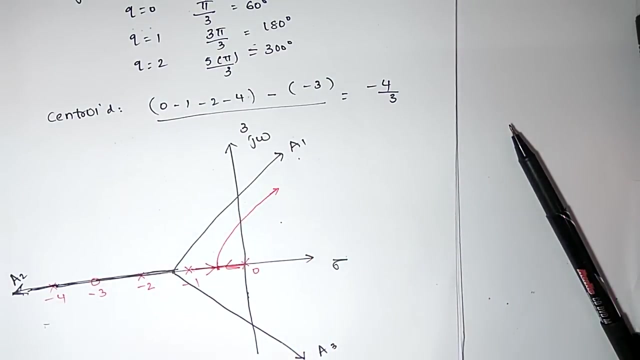 As it is an odd number, root locus exists and moves away, So it breaks. So whenever it breaks, it moves past the zero point, It moves parallel in the direction of azimuth. So this is the direction of the root locus. So this is the another direction of the root locus branch. 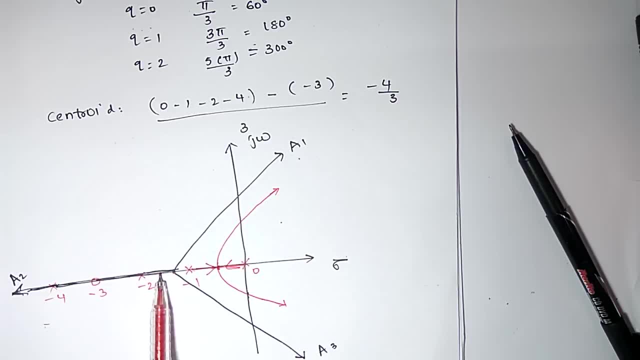 Next, between minus 1 and minus 2, root locus does not exist. As you take any point between this, on the right hand side of it, it exists even number of poles. So root locus does not exist. And between minus 2 and minus 3, there exists odd number of poles, which is 3 poles. 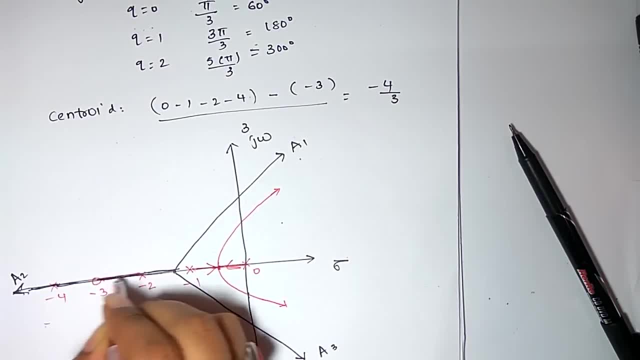 So root locus exists, which moves away from a pole and moves towards a pole 0. And again between minus 3 and minus 4, again, root locus does not exist, As the sum of poles and zeros on right hand side is even. 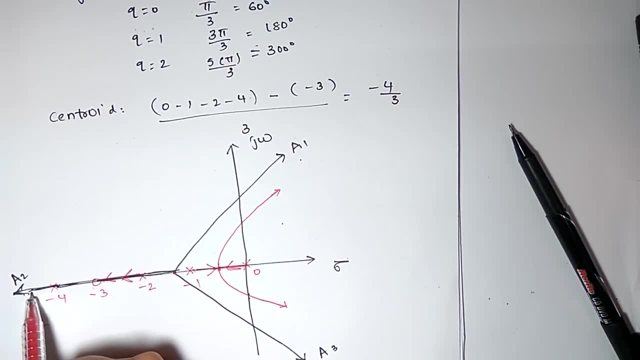 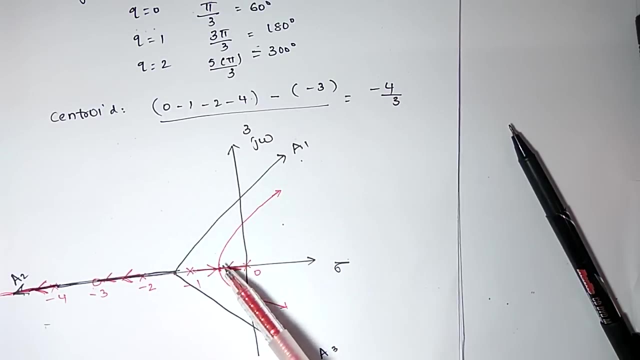 1,, 2,, 3, 4.. 4 is even. So, if you take this point, root locus exists and moves away from the pole. So if you want to calculate, you can calculate the gain at the breakpoint. 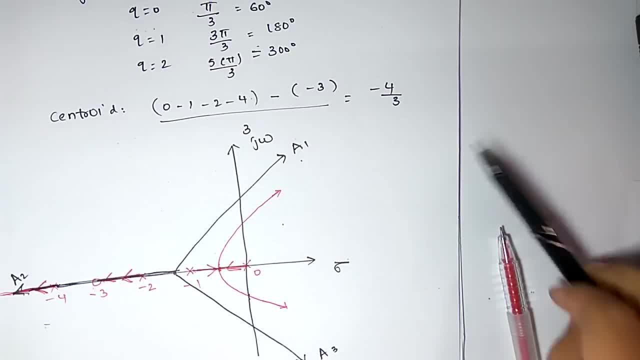 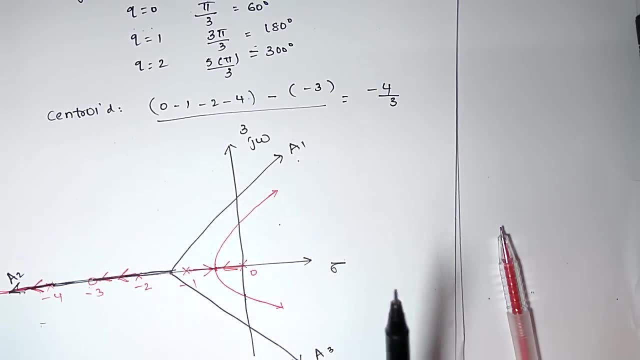 You can calculate the breakpoints dk by ds. Otherwise, simply, if they ask just to sketch, then you can leave like this, Because finding the breakpoint in this case will be difficult because it is a higher order system, So you cannot get the roots easily. 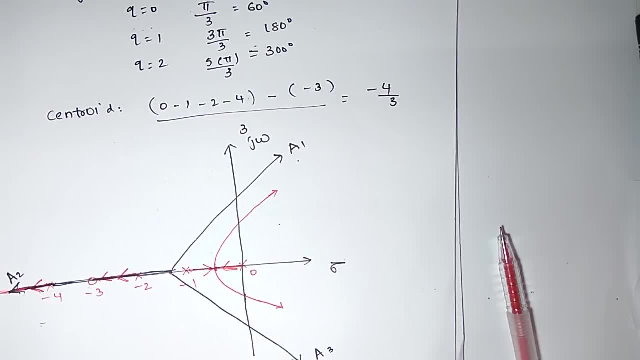 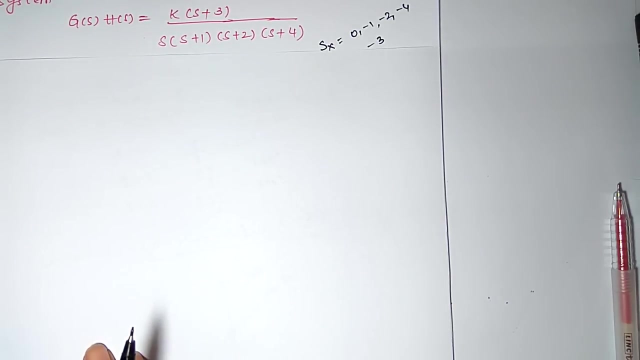 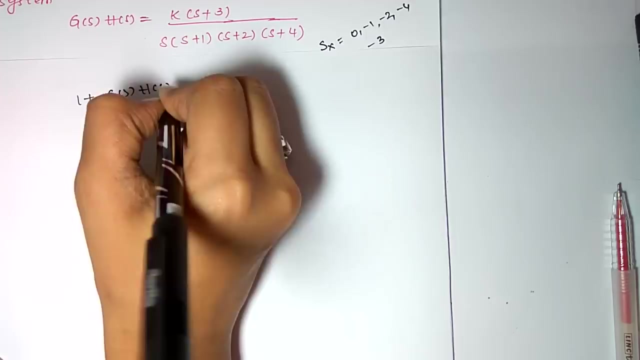 If you want to find the point of intersection at this point, So you can find that using the R-H criterion, So that we can see now here. So first we need a characteristic equation to tabulate R-H criteria. The characteristic equation will be: 1 plus g of s. h of s is equals to 0.. 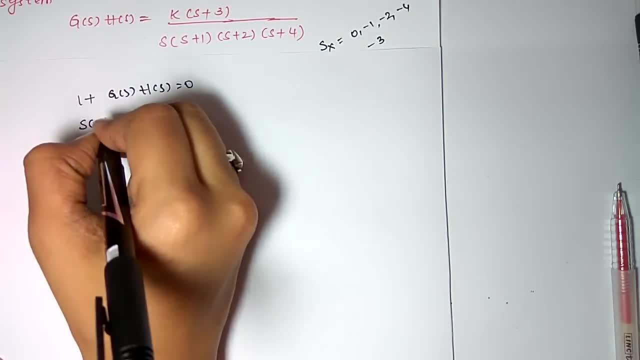 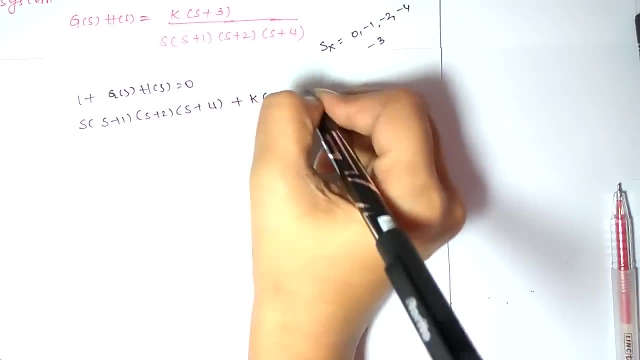 So given g of s into h of s, using that you can get s into s plus 1, s plus 2 into s plus 4, plus k into s plus 3. It equals to 0. So you can get the characteristic equation. 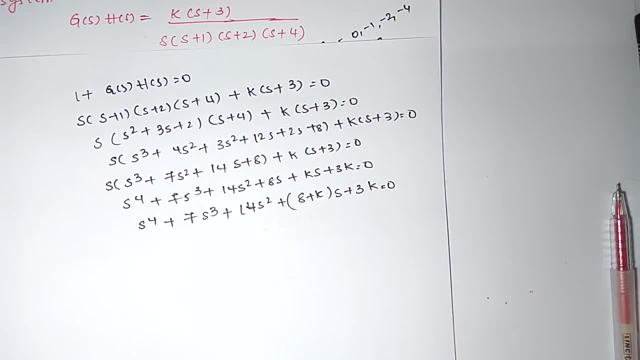 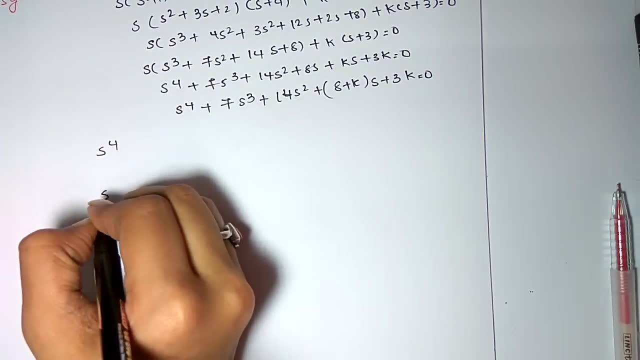 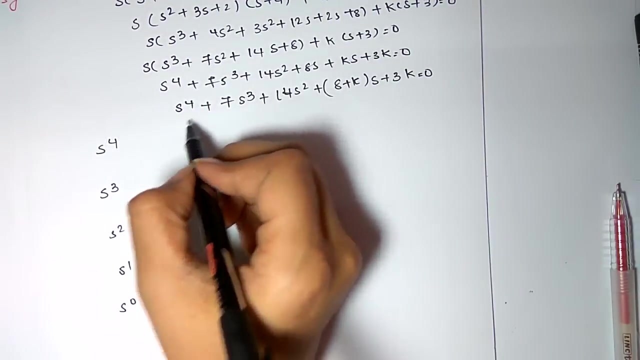 So this is the characteristic equation And you can now generate the root table s power 4, s cube s square s power 1, s power 0, s power 4.. Start with the even coefficient and alternatively 4,, 1,, 14.. 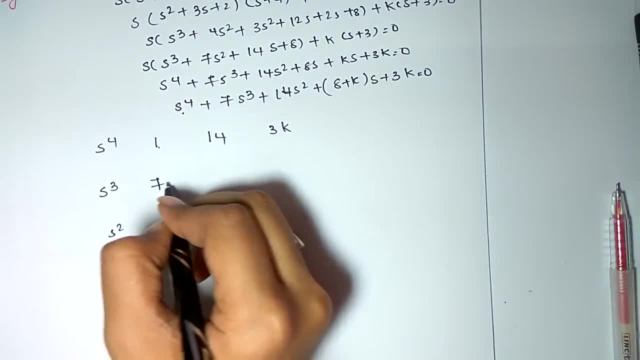 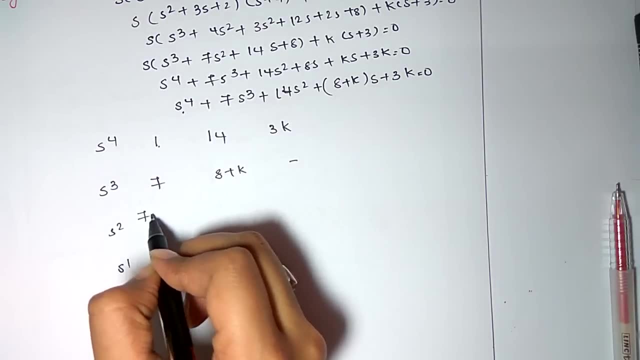 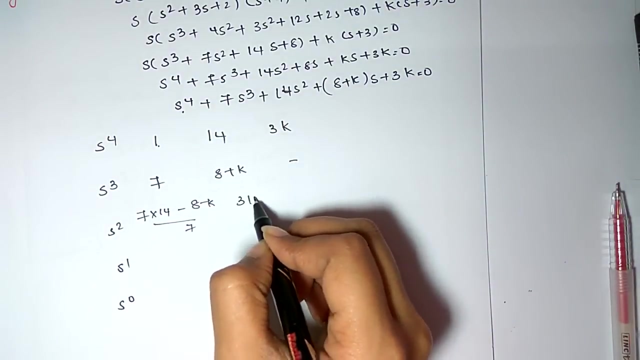 And 3, k, And this is 7, 8 plus k And this is nothing: 0.. So 7 into 14, minus 8 minus k by 7.. 7 into 3k, 0 by 7, 3k. it is. 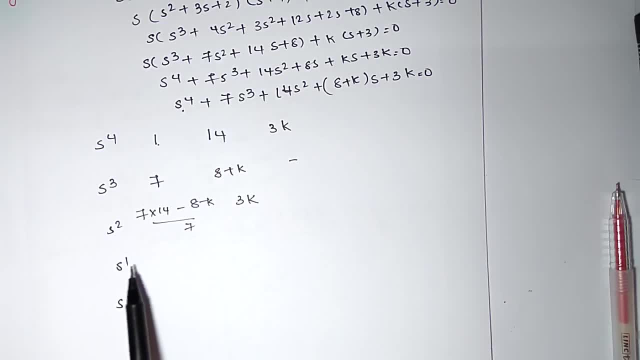 So, as we know that always, if anything, if the root locus crosses the imaginary axis, it means it is marginally stable. That means, if the system has to be marginally stable, that means one of the rows should be completely 0.. 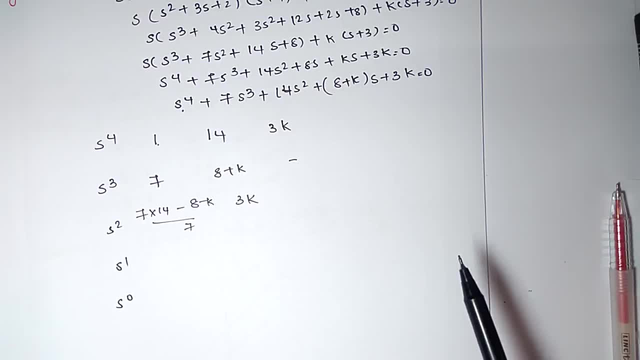 And already we have discussed that, that the row will be completely 0, that will be odd number, Which has odd number of s. That means this row will be completely 0.. So to get this row completely 0, what should be the value of k? you can find: 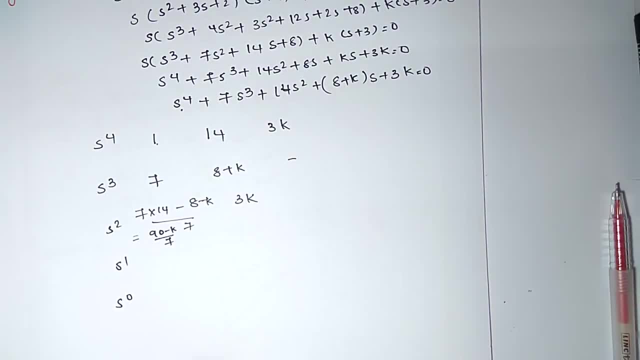 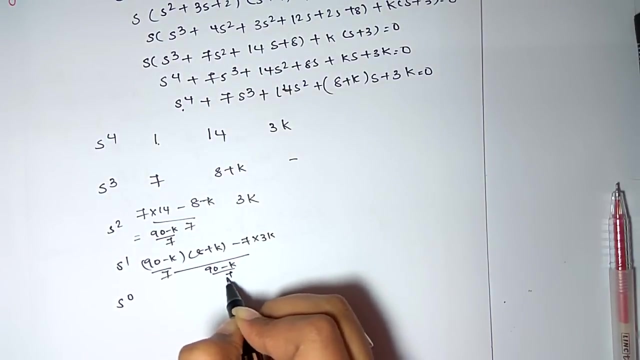 So 7.. So which will be equals to 9.. 90 minus k into by 7, into 8 plus k minus 7 into 3k by 90 minus k by 7, 0.. 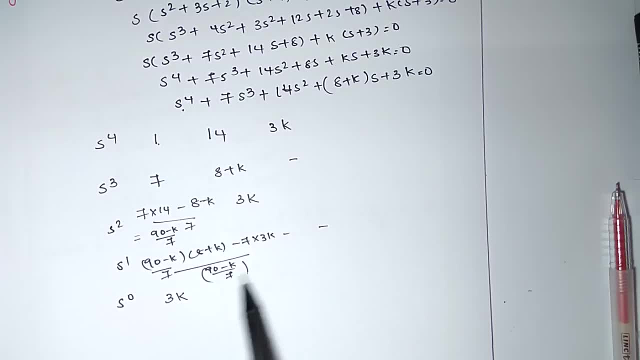 So this is 3k, So you can equate this equation to 0 and you can get the value of k For which it is the system will be crosses the imaginary axis, So you can get it as: 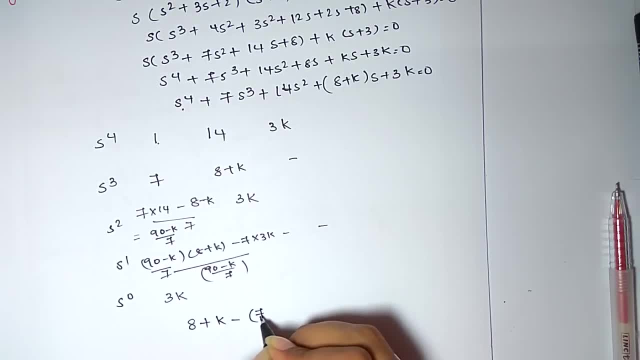 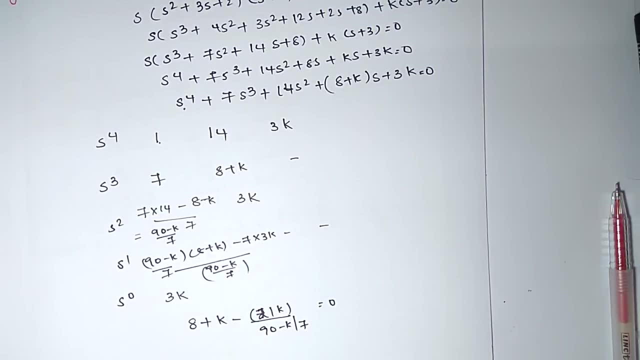 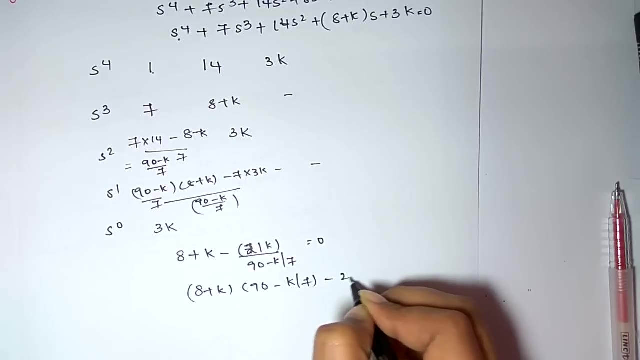 8 plus k minus 7 into 3k, which is 21k by 90 minus k by 7, is equals to 0. So 8 plus k into 90 minus k by 7, minus 21k, equal to 0.. 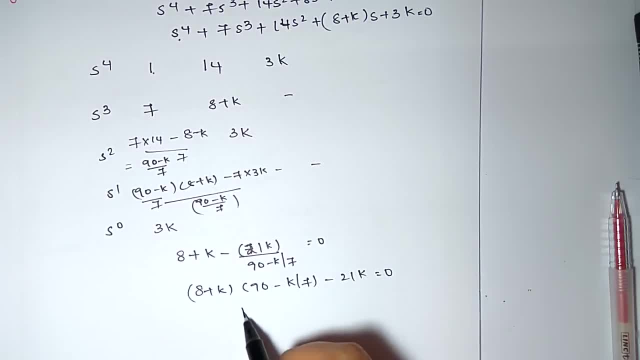 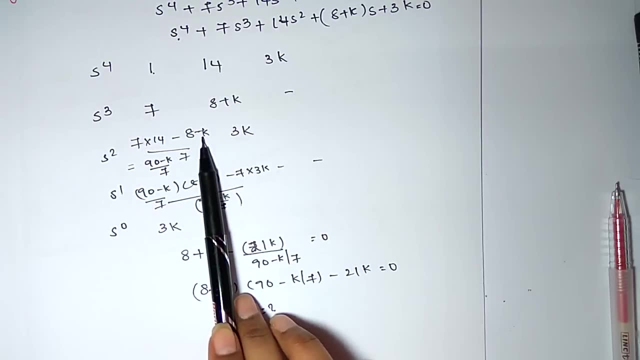 If you can simplify this equation, you can get the value of k For which the system crosses the imaginary axis, And if you can substitute here The k value and you can get the value of the root also. So if it is asked in the question, you can do in this way.